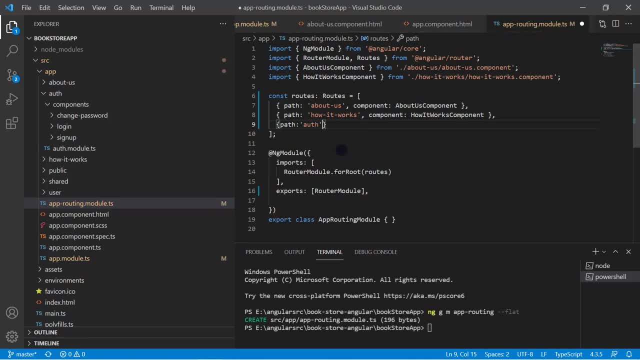 is the basic keyword and I can define that over here: auth. Then we have to define the component And this component is basically a layout for this particular path And in this auth we do not have a separate layout. But as of now, if your layout is same, then you can use this app component. But if your 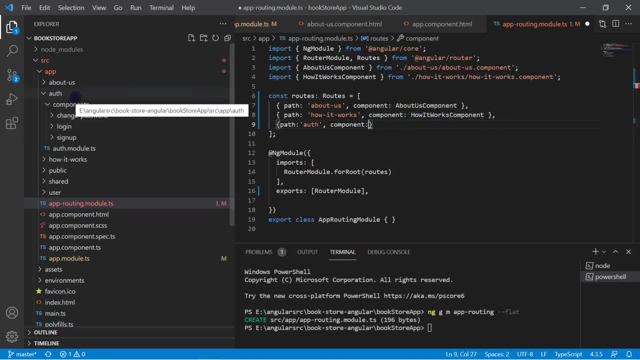 layout is different, then you can generate one more component in this auth And you can use that component over here as a layout. Let's generate a new component over here. So here I'm writing ng, g, c And I want to generate a new component inside this auth. 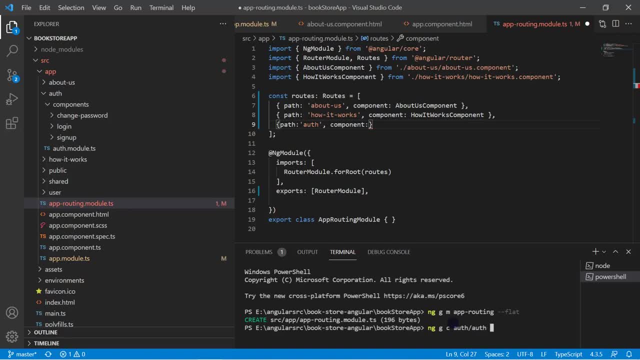 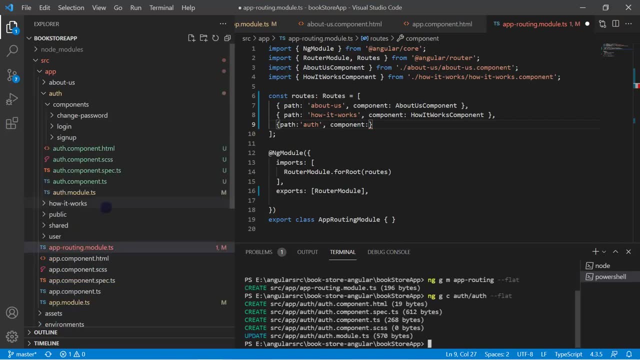 Let's say, the name of my component is also auth, And this time I do not want to generate the parent folder, So basically I want to have only the flat files. Hit the enter button And here you can notice that along with this auth module we have this auth component as. 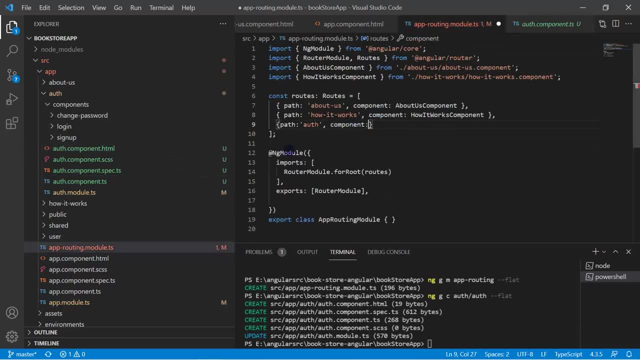 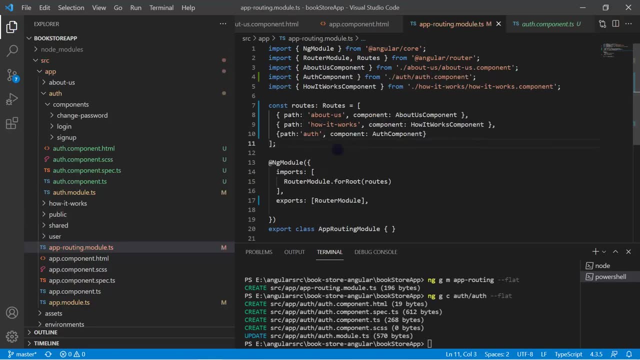 well, So let's copy this auth component, Go back to the app routing module And over here let's define this auth component. And remember: this time we are defining the path for a separate module and that is the auth module, So for that we have to write one more property. 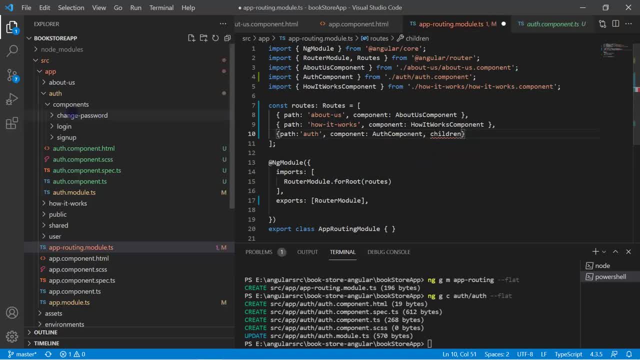 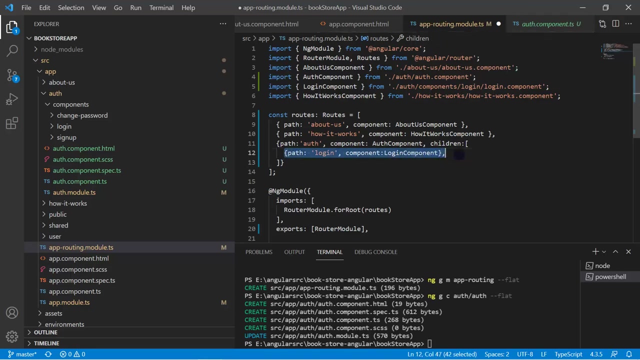 over here And that is the children. This is because all our components are available in this auth module And again the similar structure. So the path this time: if it is login, then I want to call the login component like this: just put a comma and copy this entire code, paste it. 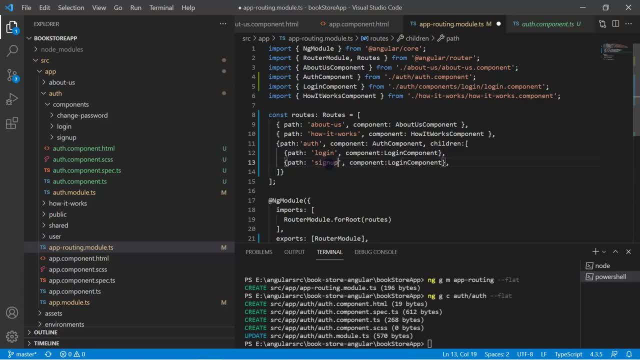 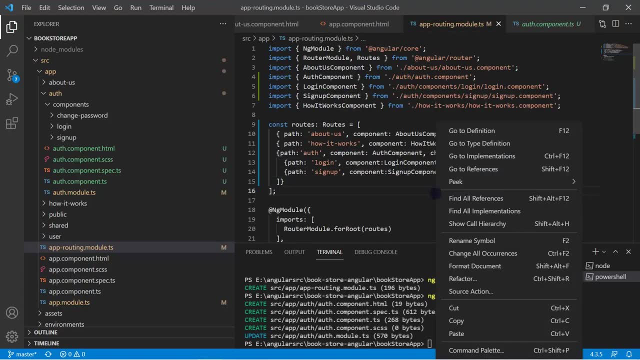 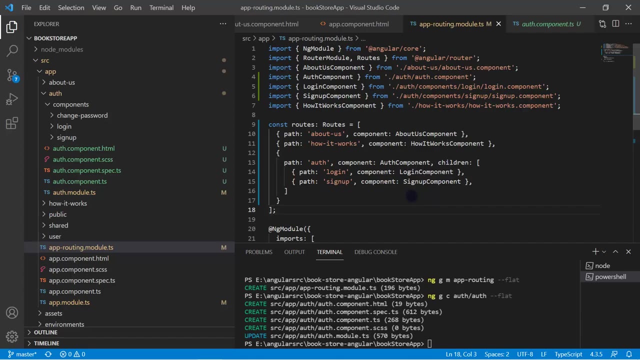 again. If it is signup, then I want to call the signup. Just save the changes, right click on this page and use this format document like this. Now let's see what are the changes in this application and how it will work on the browser. There is no change on this home. 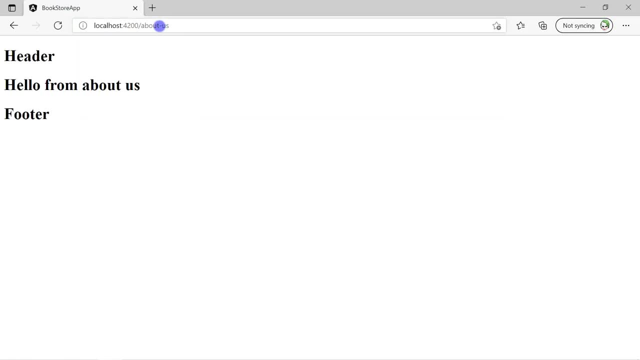 page and about us is also working fine. Let's see for the how it works. It is also working fine. But this time if I want to access the login page then I have to write auth and then the login, Hit the enter button And here you can see that still we are getting.